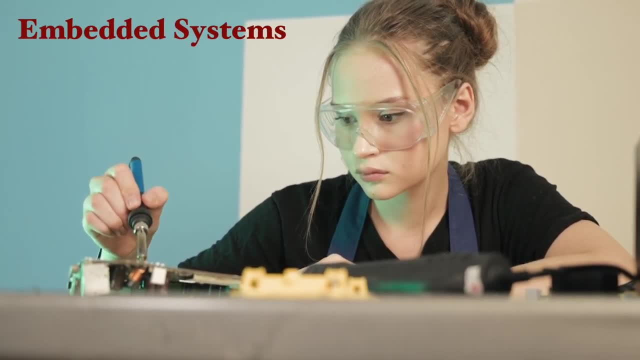 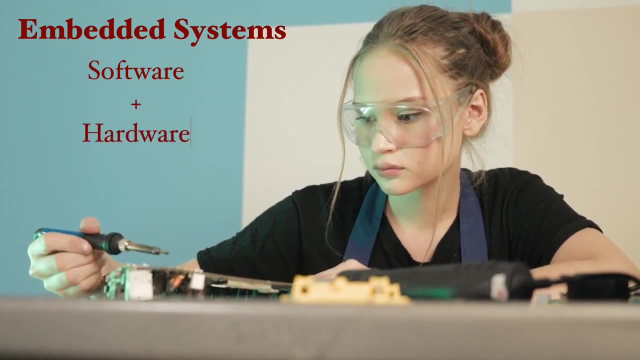 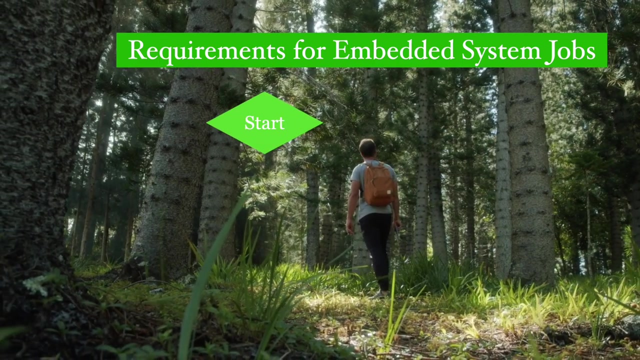 Embedded systems are highly diverse field that encompasses both sides of electronics, software and hardware. This diversity can often create chaos, leaving many aspiring engineers wondering what exactly they should study to break into embedded system companies. But fear not, this video is here to provide you all with all the knowledge you need from the very beginning. 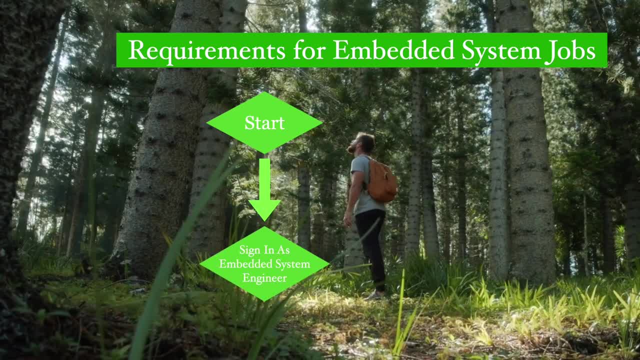 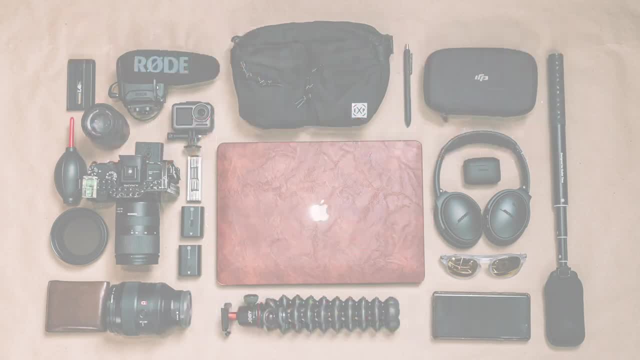 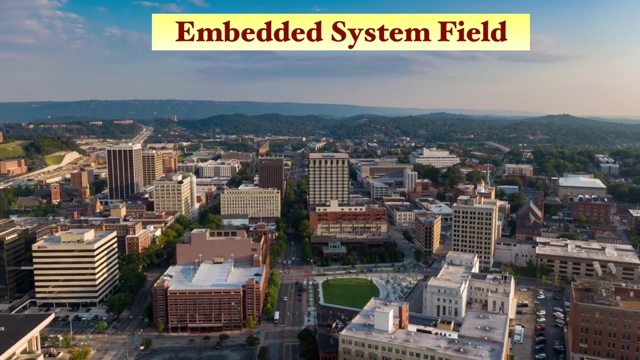 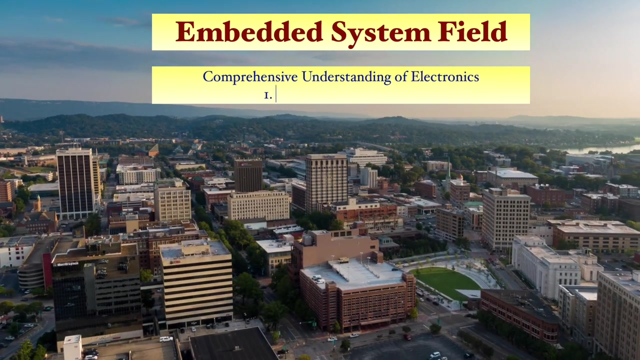 to signing on as an embedded system engineer at top companies. So let us get started. Every job has a set of requirements, and the field of embedded systems is no exception, With its diverse nature. embedded system jobs demand a comprehensive understanding of electronics, combining both hardware and software expertise. However, as a facer, 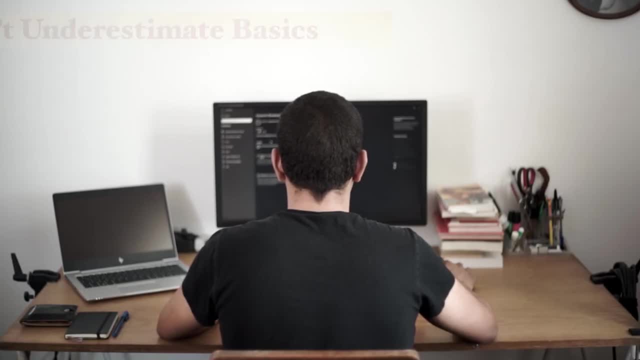 it is natural not to have extensive practical experience In such cases. interviewers often evaluate candidates based on their fundamental knowledge of electronics and their problem-solving skills. As a facer, it is natural not to have extensive practical experience In such cases. interviewers often evaluate candidates based on their fundamental knowledge of electronics and their problem-solving skills. 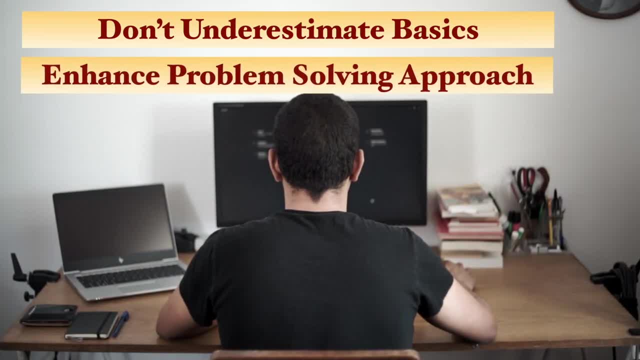 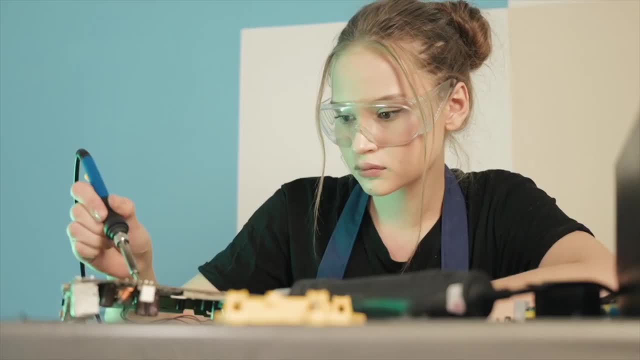 As a facer, it is natural not to have extensive practical experience. Therefore, aspiring engineers aiming to work in the embedded system field must cultivate these qualities. In this video, we will start by exploring the hiring process and use that as a foundation to conclude the requirements for becoming an embedded system engineer, The primary focus. 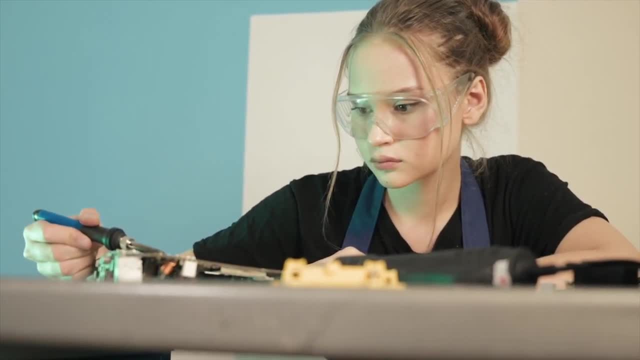 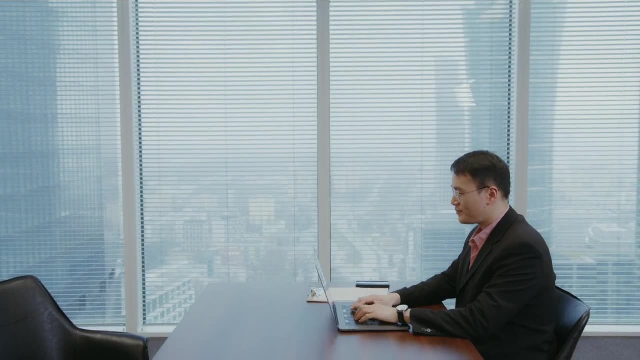 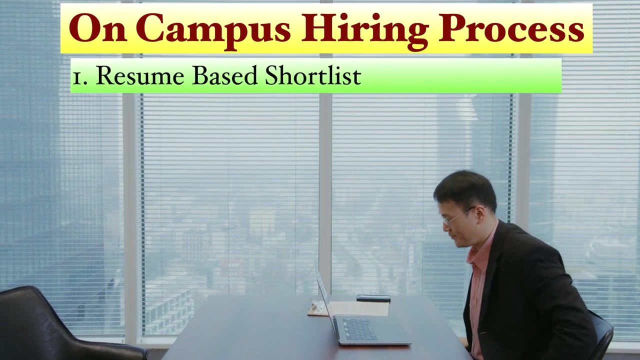 will be on the knowledge necessary to secure opportunities in the embedded system companies. So let us dive in and uncover the essential knowledge needed to thrive in the world of embedded systems. On-campus hiring typically follows a four-step process. The first one is resume-based shortlist. It is crucial to tailor your resume according 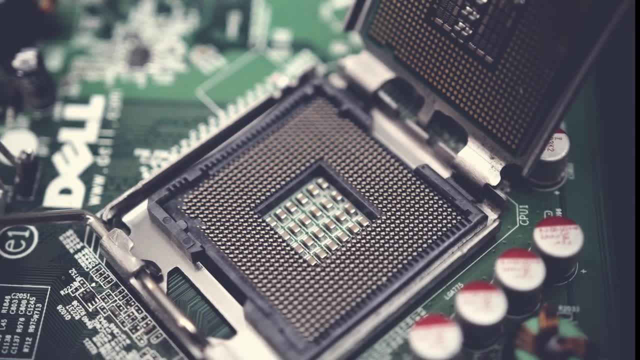 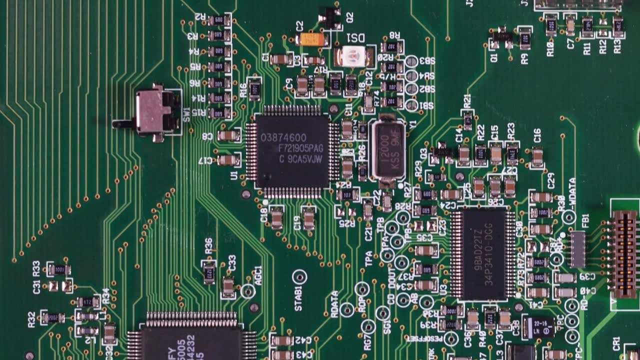 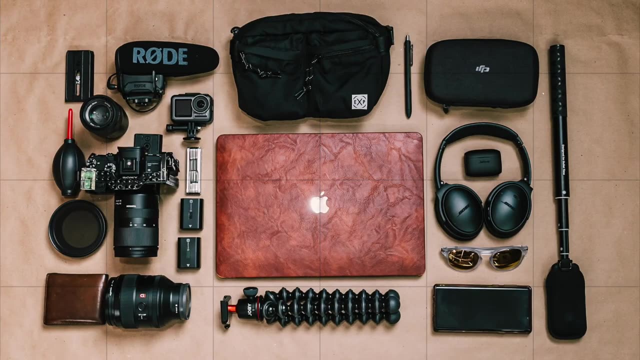 to the required skills and in this video we will discuss those skills in detail. RETURN TEST: Companies often conduct a return test with no negative marking. To clear the test for embedded system roles, it is essential to be familiar with basic electronics operating systems, basics of C computer architecture. 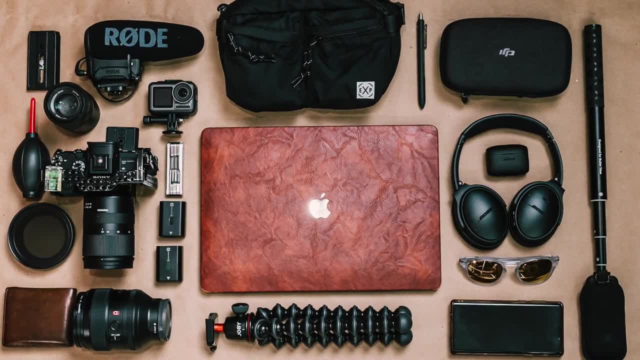 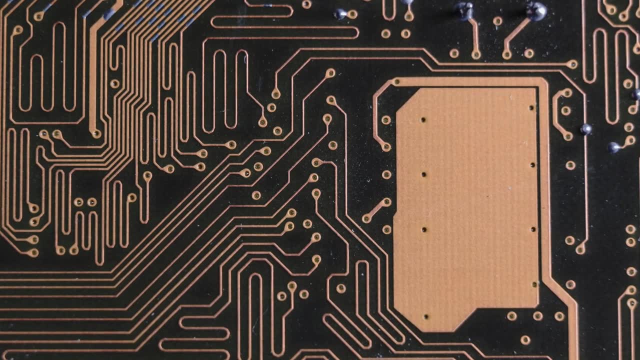 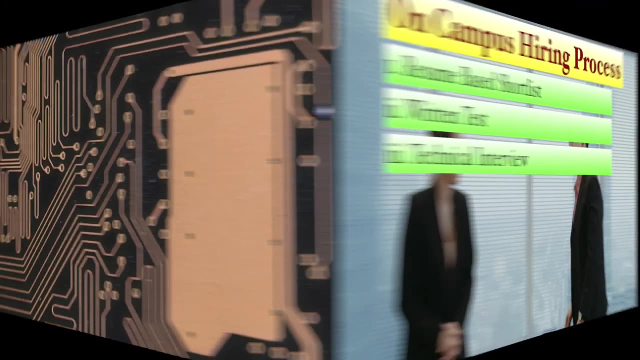 digital electronics and gate-level aptitude questions. Technical Interview. In this section we will delve into the specifics of clearing the technical interview for embedded system roles. We will cover the key areas of knowledge and provide strategies to excel in this crucial step. HR Interview. The HR interview usually involves basic questions. 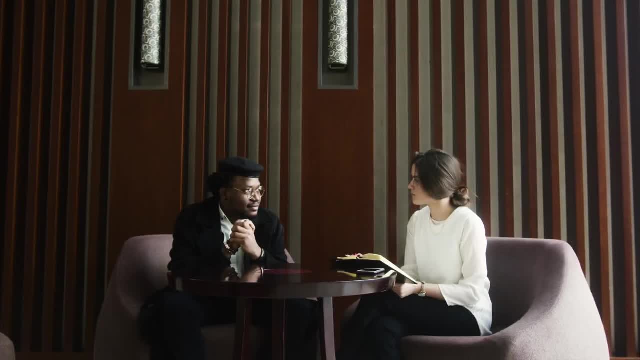 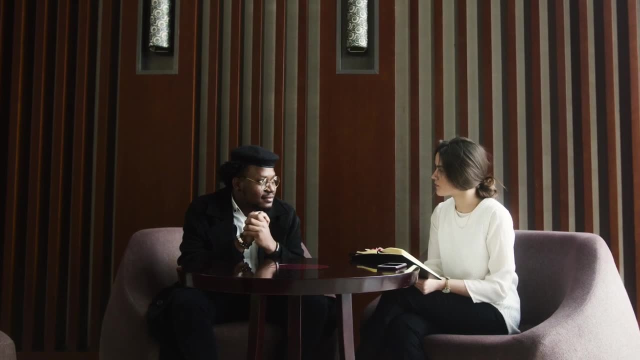 about why you are interested in the company and your preferred location. These questions can easily be answered and we will briefly touch upon them. The main focus will be on formulating strategies for the second and third steps, which are return test and technical interview. 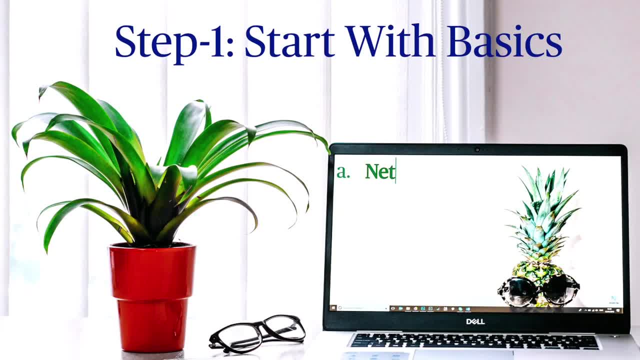 The first and fourth step is to prepare yourself for the helpful, accessible interview. Start with the basics. Network theory is a fundamental building block for electronics engineers. It provides the necessary foundation to understand advanced subjects. Begin by familiarizing yourself with the basic circuit analysis authorities, such as KCL and KVL. 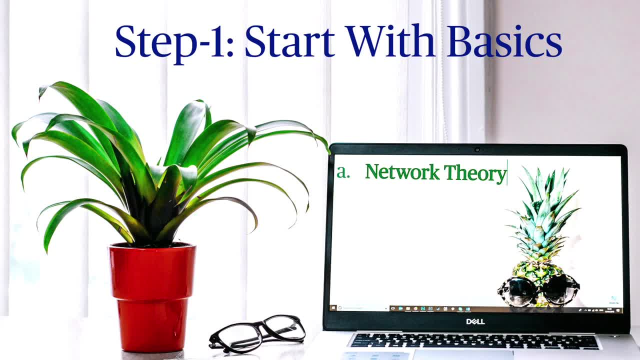 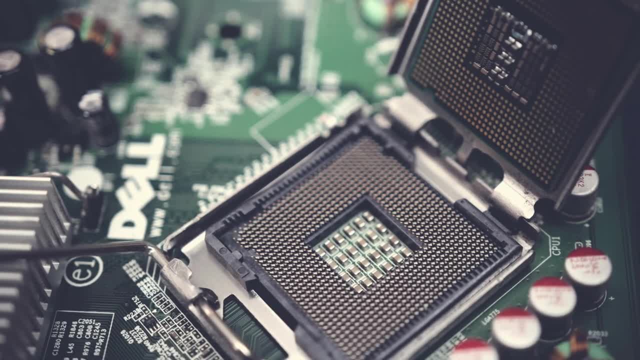 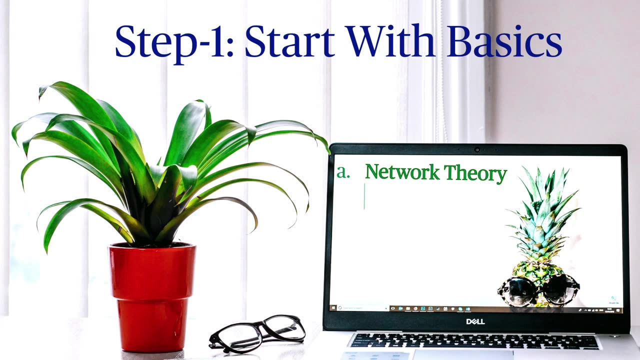 Additionally learn about various theorems and pay particular attention to RLC circuits. To gain a solid understanding of network theory, you can utilize gait coaching lectures specifically designed for these subjects. so in this way you can prepare network theory and it is a must-do subject for qualifying in written test. second basic subject is: 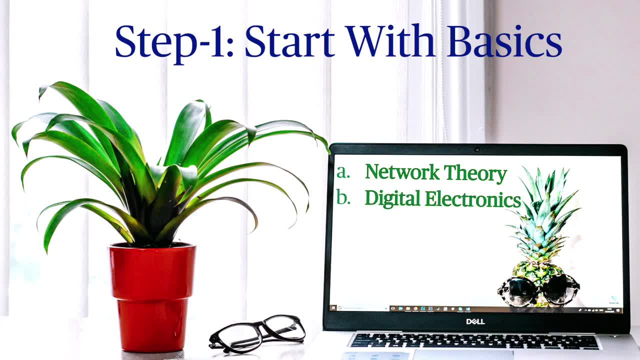 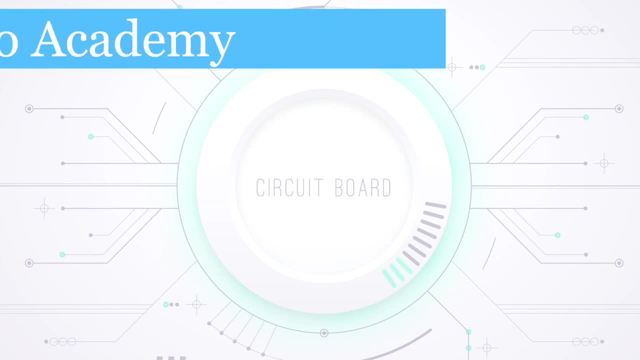 digital electronics. there are numerous valuable and free online courses available to learn from a start, with topics such as Boolean algebra and progress to combinational and sequential circuits. so some of the very popular courses are digital electronics by Neso Academy. second one is Sujaya sir's. 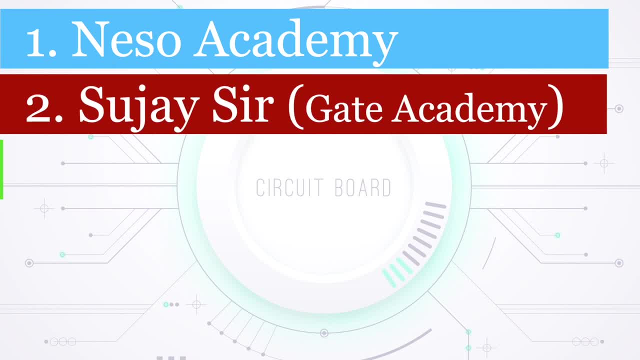 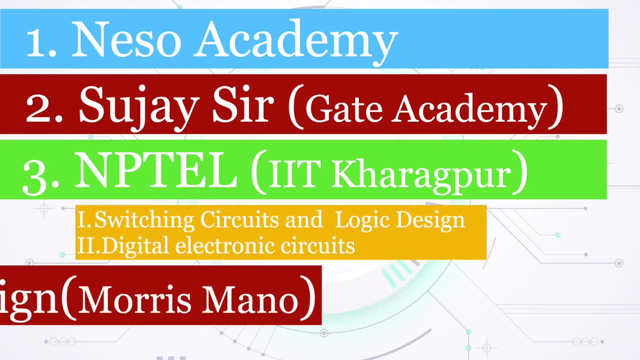 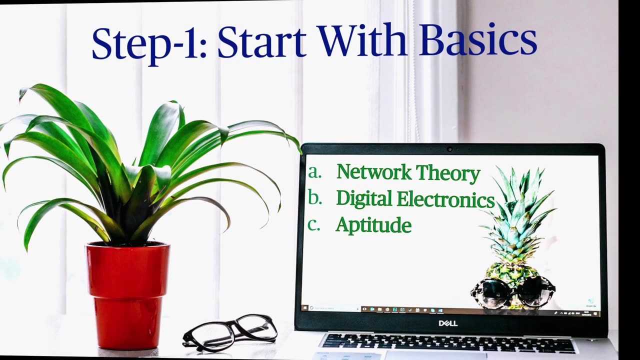 lectures. who is a teacher in gate Academy. if you want a more practical perspective, then consider the digital electronics course by NPTEL IIT Kharagpur, and also the digital design book by Morris Manu. finally, the third area to focus on is aptitude as an engineer. you are likely already familiar with. 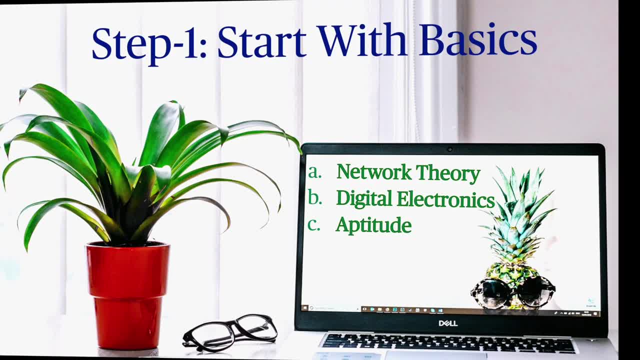 fundamental mathematics. so following any gate level aptitude course should enable you to solve gate level aptitude problems. please note that I have provided the links to the courses in the description for your convenience. so this was all for today's video. thank you for watching and see you in the next video. 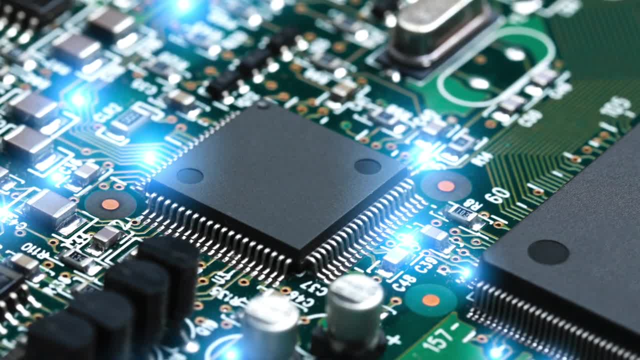 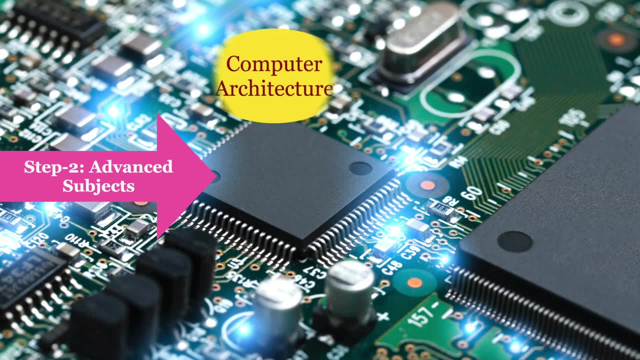 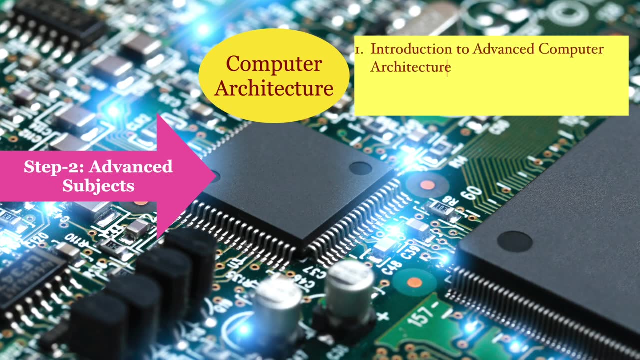 all about the first step. now let's go to the next step, the preparation of advanced subjects. one crucial area to focus on for embedded system interview is computer architecture and organization. I recommend taking the course introduction to advanced computer architecture offered by NPTEL IIT Kharagpur. this course provides both theoretical and practical understanding. 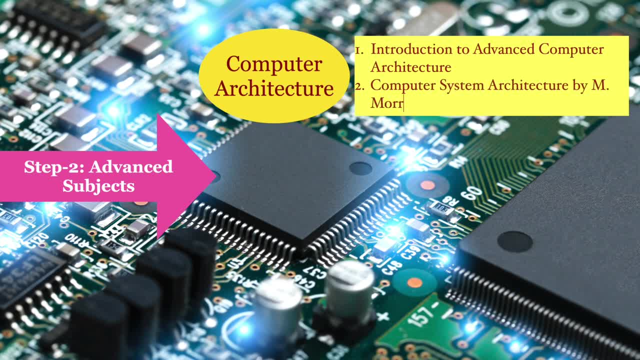 of the subject. to supplement your learning you can also refer to the book computer system architecture by Morris Manu. as the NPTEL course is extensive, it is important to prioritize the following topics: microprocessor and microcontrollers. start with the basics of 8085 microprocessor and 8051 microcontroller. other significant areas covered in the 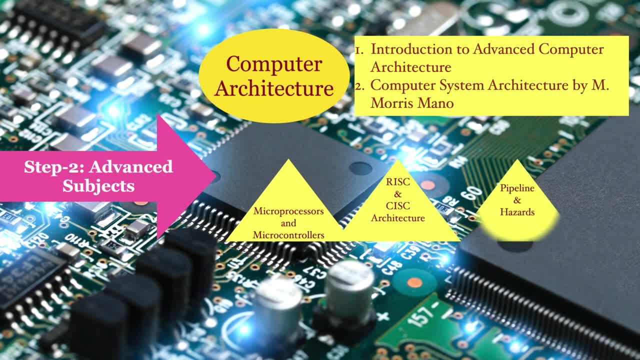 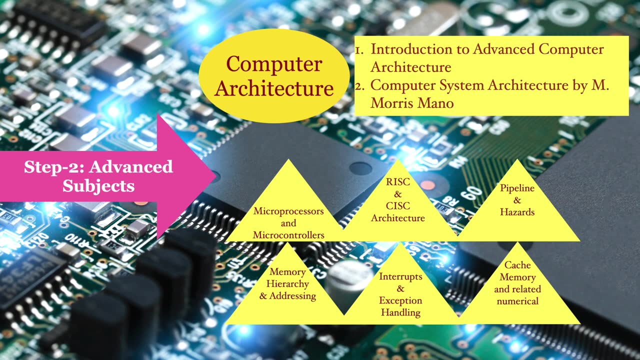 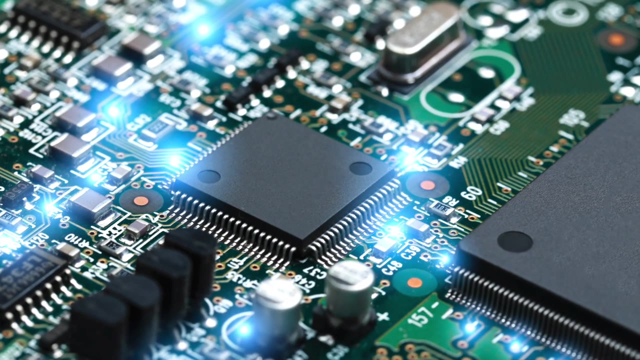 course include risk and sys architecture, pipeline and hazards, memory hierarchy and addressing interrupts and exception handling, HM memory organization. ensure that you have a strong command of these topics to excel in embedded system interviews. so this is very much important subject for embedded system interviews and also it will be required when you will be doing your embedded 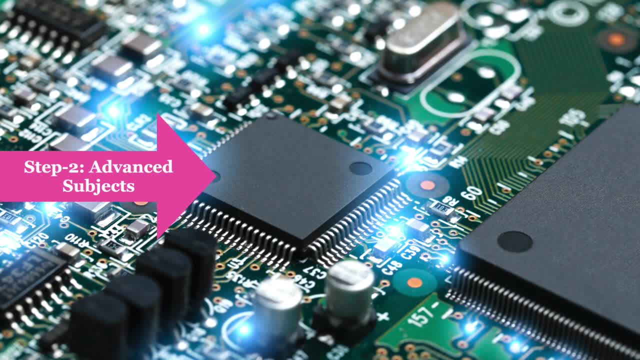 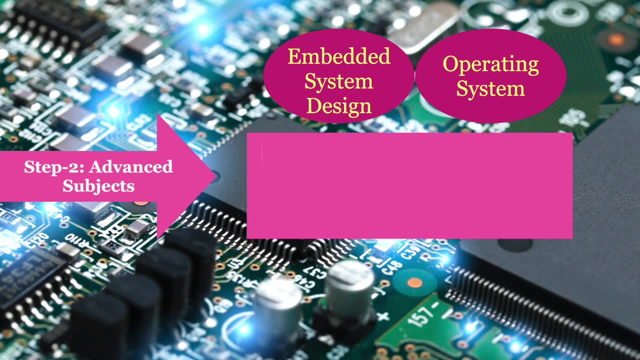 system job. so the next advanced subjects are embedded system design and operating systems. so here are some recommended resources. are operating systems? Java inserts lectures freely available on YouTube, provide a comprehensive coverage of operating systems. you can search for his lectures to access the relevant content. second one is this: 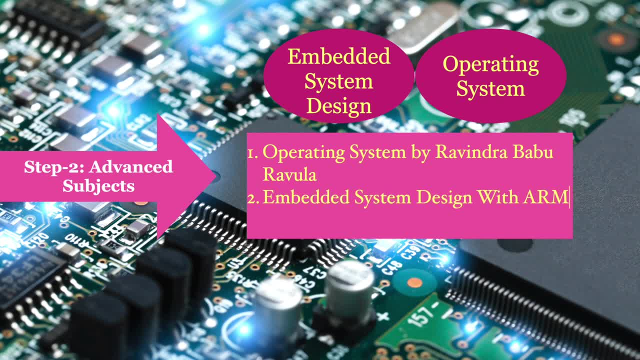 course includes a involving lecture on what is embedded system for students status information on the list at the top: toела letter on This course focuses on embedded system design utilizing ARM architecture. It provides valuable insights into the design and implementation of embedded systems. 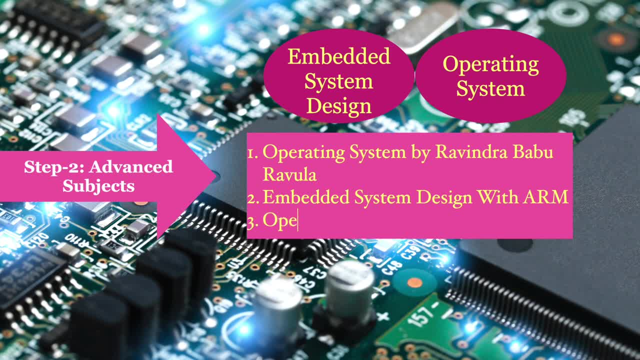 You can find the course using the provided name, And there is one more course from the Naso Academy on Operating Systems. Watch few lectures from both Naso Academy and Ravenser series and decide which one resonates with your learning style. Make sure to cover the following topics in your study: 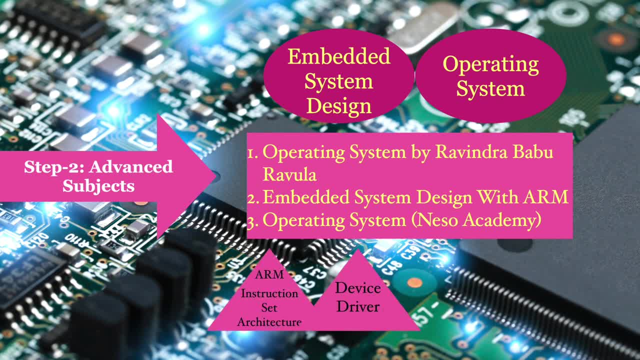 ARM Instruction Set Architecture Device Drivers. So learn about the device drivers, which are the software components that drives communication between hardware devices and the operating system. Device drivers play a critical role in embedded systems. Third topic is Basic of Communication Protocols. Gain knowledge about common communication. 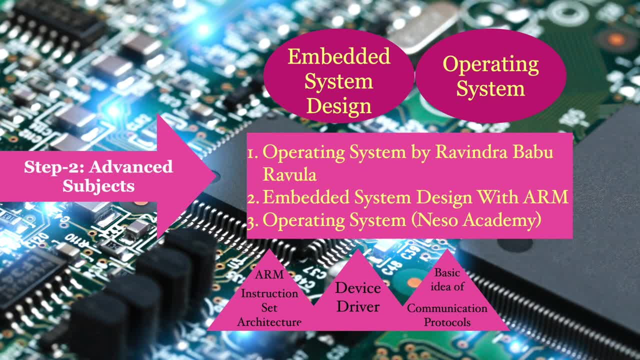 protocols such as I2C, SPI, UART and others. These protocols are frequently used for inter-device communication in embedded systems and usually asked in embedded system interviews. And there is one more important topic from operating system that is Processed Scheduling. Study the concepts of process scheduling, which involves managing and allocating system resources. 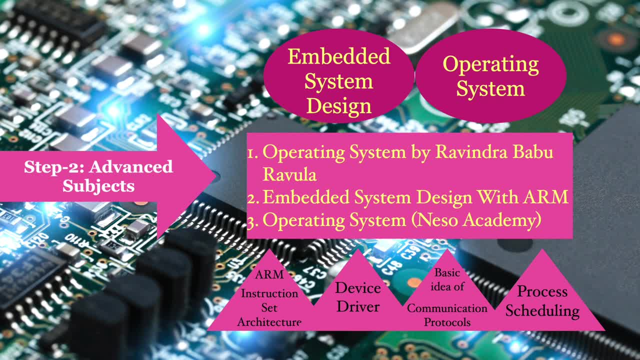 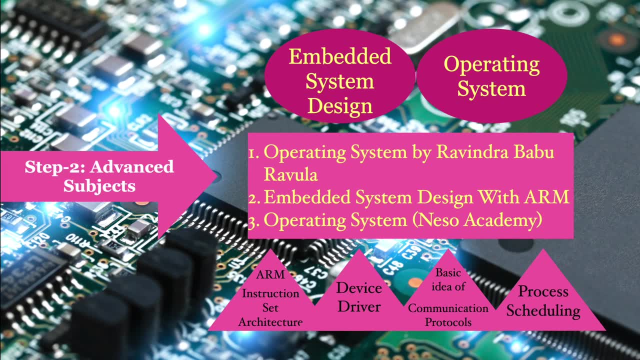 to different processes in an operating system. Ensure that you dedicate enough time to these topics to develop a strong foundation in embedded system design and operating systems. As we progress through the roadmap, learning programming aspects is indeed crucial, And it can be done in parallel with the previous step. 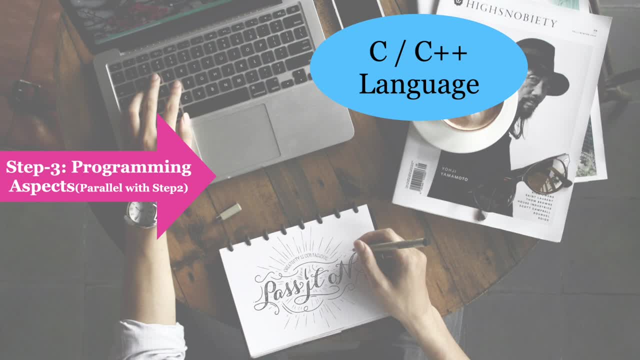 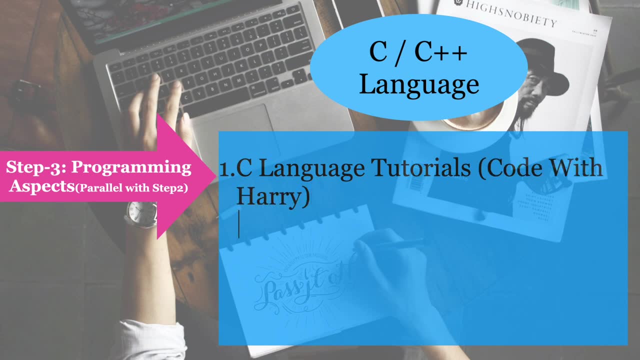 C and C++ are fundamental languages to learn and there are numerous courses available to help you get started. Here are the some recommendations. While going through above courses, pay special attention to topics like data types, loops, arrays, pointers, memory allocation, searching, sorting and storage classes. 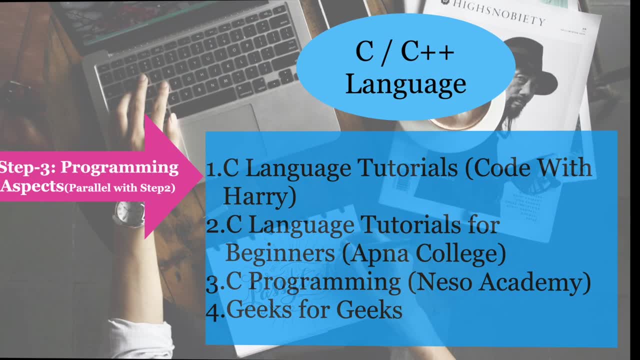 These topics are essential for building a strong foundation in programming in respect to embedded system jobs. So remember, C is particularly important for embedded systems, so ensure that you complete these courses and get a solid command over the mentioned topics. The final step involves fulfilling additional requirements. 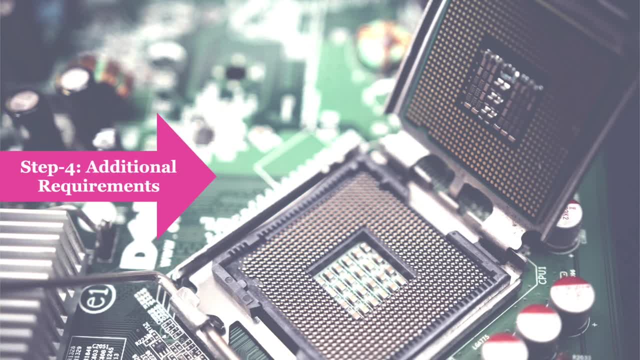 That may be sort of tasks. For example, you may need to complete a course on programming. It's recommended to think about the type of tasks that you are working on and what you are doing in that particular course. This is considered by companies working in both embedded systems and VLSI design, such 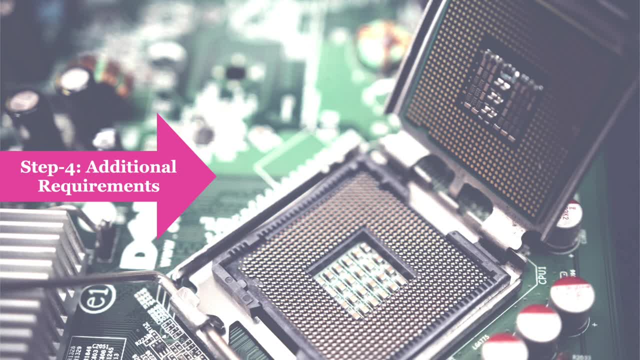 as Qualcomm, ARM, Western Digital and Texas Instruments. These companies often expect candidates to have knowledge of chip design concepts in addition to embedded systems. To address these requirements, consider the following suggestions, And the first one is opt for a VLSI design elective in your final year of graduation. 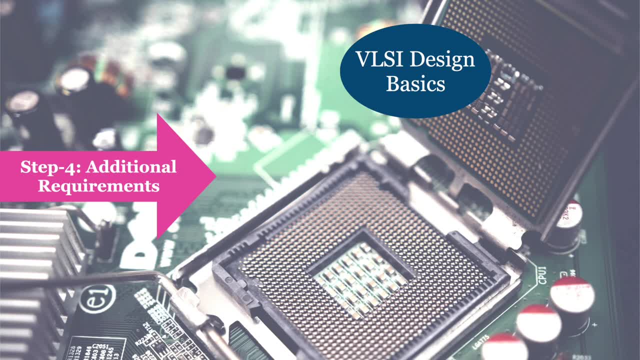 This will allow you to gain a deeper understanding of chip design concepts and hardware description languages such as Verilog and other relevant topics. Let's consider the following: By choosing this elective, you can prepare yourself for questions related to chip design during embedded system job interviews. 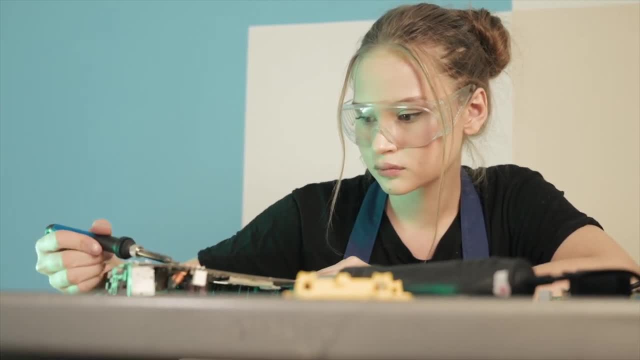 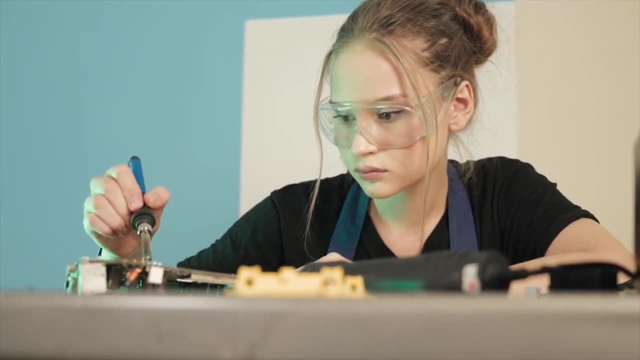 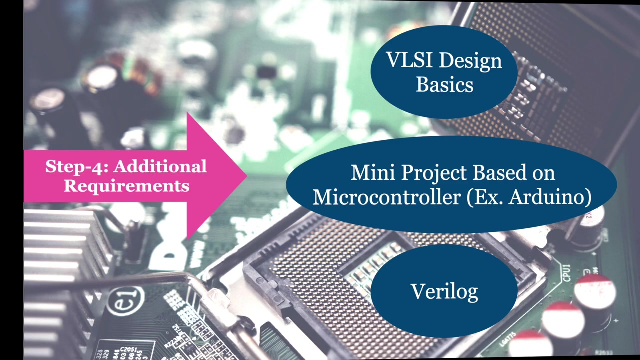 This way, you can cover both embedded systems and VLSI design aspects without any additional effort. Along with all these subjective knowledge, one should have practical exposure as well. So while selecting your final year project or Mtech thesis, remember choose a project. 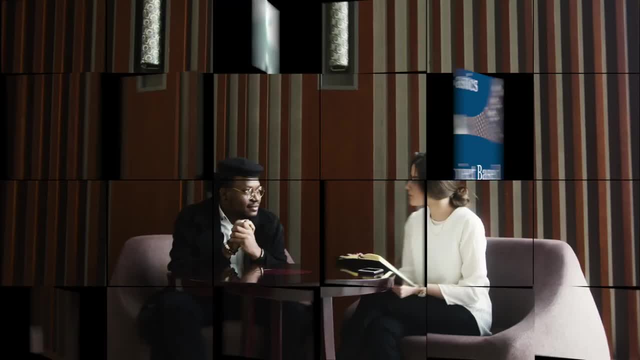 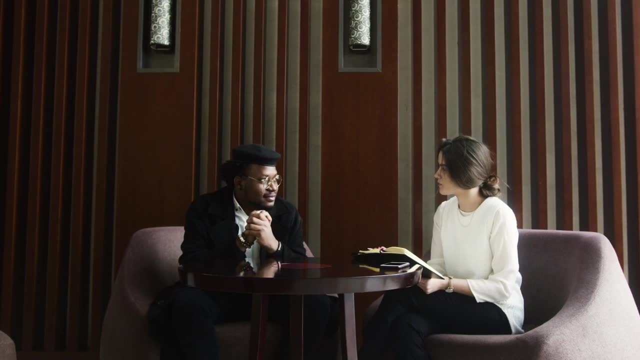 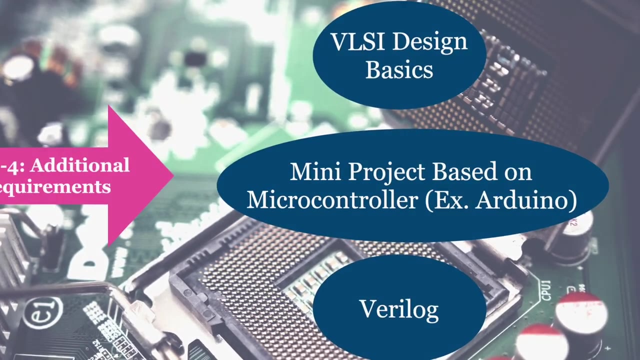 that focuses on microcontrollers or any other embedded system related area. By working on such a project, you will gain practical experience and develop skills that are valuable for an embedded system profile, So this project will enhance your resume and demonstrate your completeness in embedded system.